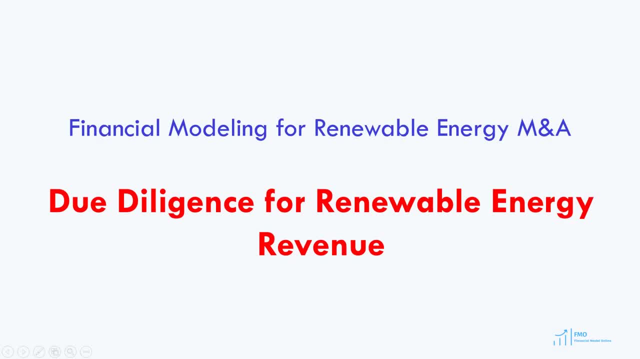 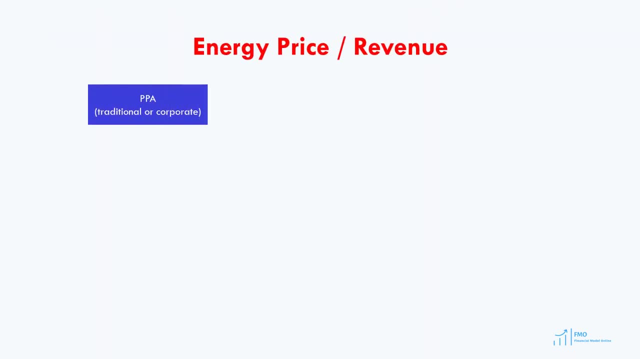 Welcome back. In today's lesson we'll focus on the due diligence for the project's revenue. One of the most prevalent payment mechanisms for renewable energy projects is the Power Purchase Agreement, or PPA. Over the past decade, we've seen a development of a variety. 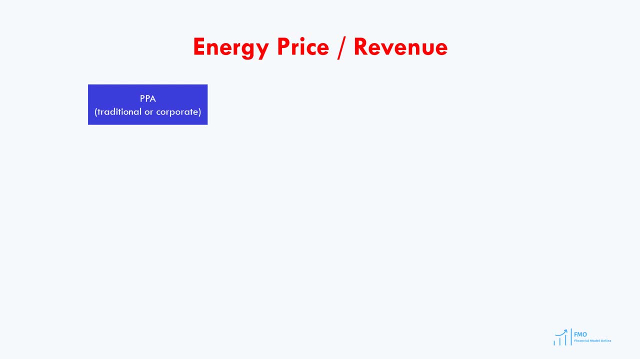 of PPA mechanisms to serve the different needs of power producers and energy consumers. Under the traditional PPA agreement, the power producer sells power directly to the utility, which then sells it to the end consumer. However, we also have a corporate power purchase. 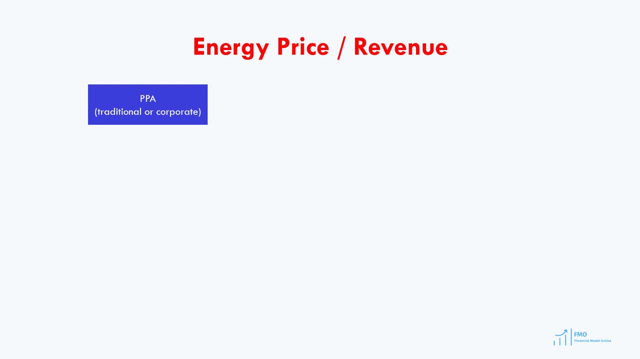 agreement where a corporate entity, not necessarily a utility, serves as the buyer. The corporate PPA can be both physical or virtual or synthetic PPA. The main features of these power purchase agreements is their long-term contractual nature, which offers a fixed price and provides 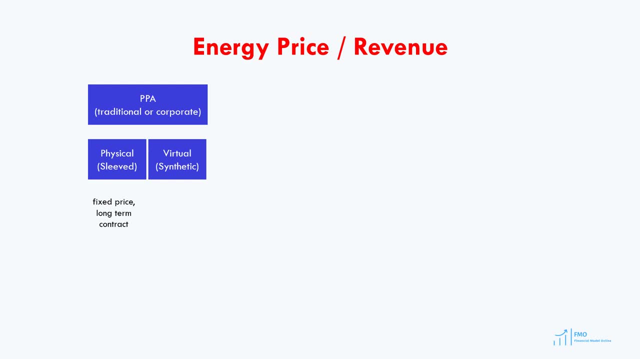 project investors and lenders visibility in output pricing and output volume. This feature is essential under project financing because if we lack price certainty, it becomes challenging for greenfield renewable energy projects to secure debt and equity financing. The virtual PPA essentially functions as a contract for difference: The power is sold. 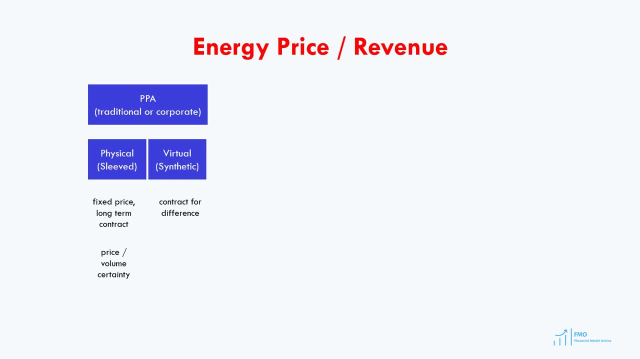 to the market, and any disparity between the market price and the PPA price is compensated by the buyer. Another important source of benefits to the power producer is government subsidy. Subsidies play a crucial role in power production and they play a key role in the development of. 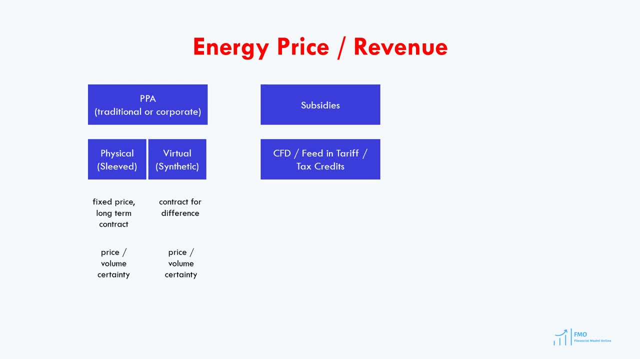 greenfield renewable energy projects. However, the government acts as a counterparty. This arrangement constitutes a subsidy, as the government guarantees a fixed price to projects, ensuring their financing and development. In contrast, the United States primarily employs tax credits as a subsidy for renewable energy projects. The tax credits have a significant 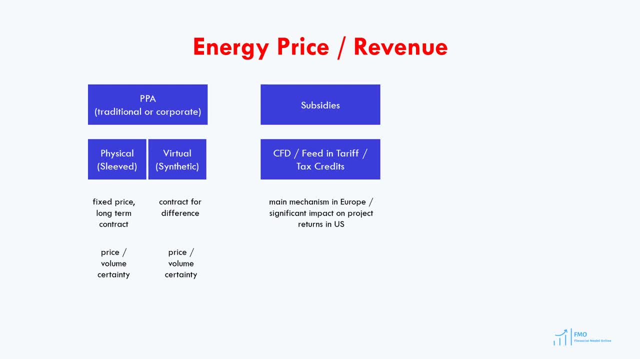 impact on project returns, as they bring about tax equity financing, thereby boosting equity returns for investors in renewable energy projects. Some projects also generate revenue through selling green attributes. Renewable energy credits are usually bundled with the energy sold under power purchase agreements. If bundled, the project will have an additional revenue stream from. 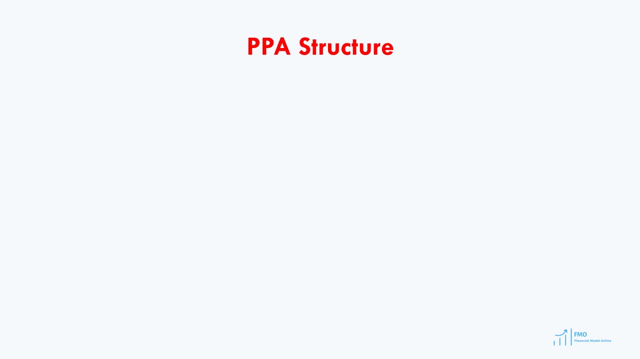 the sales of these green attributes. Let's briefly review the PPA structures prevalent in today's energy markets. First let's take a look at the traditional PPA structure. Here we've got the power producer who sells power to a utility, and then we've got the power purchaser who buys energy from the 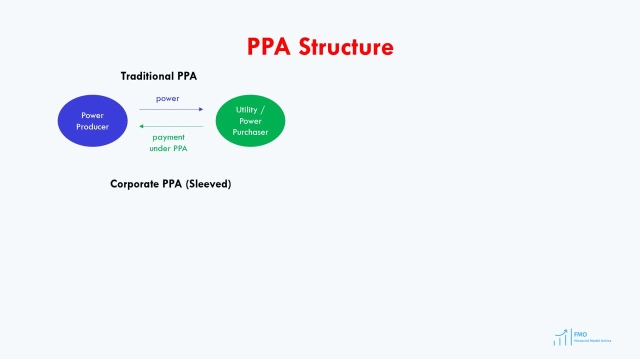 utility. In contrast, the corporate PPA involves a corporate buyer instead of a utility. Companies like Google or Microsoft, which require significant power for their data centers, can source part or all of their power. In contrast, the corporate PPA involves a corporate buyer instead of a utility. 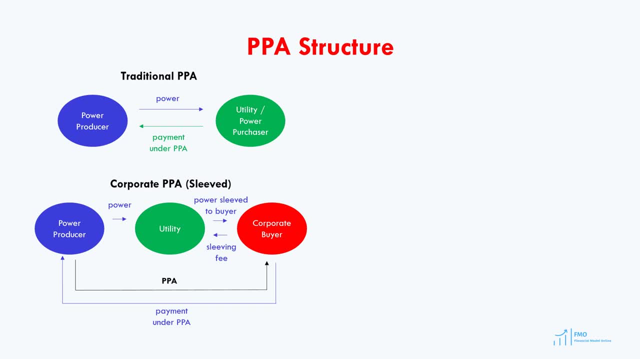 Then there are the commercial mercaries who build energy with the money experience. There are also those who who outsource their prices. Under this agreement there will be a fixed PPA price, known as the strike price. So if the strike price is higher than the wholesale price, the power producer pays the difference to. 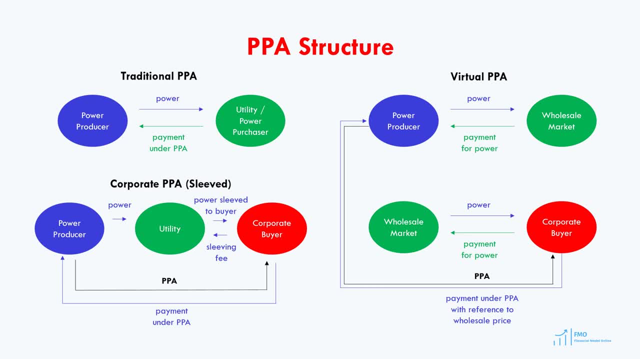 the corporate buyer. However, if the wholesale price is lower than the strike price in the PPA, then the corporate buyer compensates the difference to the power producer. In both traditional and virtual PPAs, long-term tenors are common with fixed energy prices and 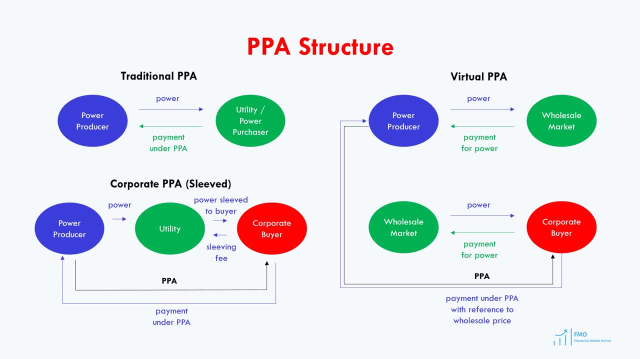 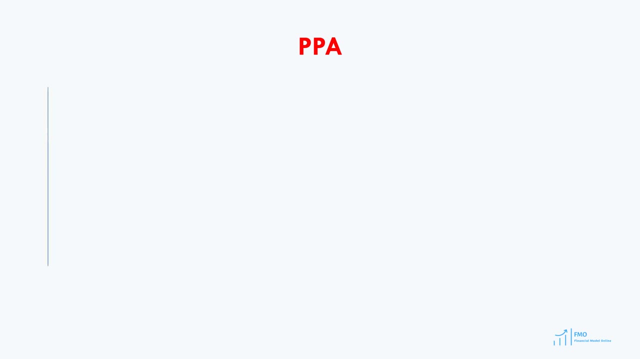 possible price escalation formulas. Typically, physical PPAs specify delivery points, unlike virtual PPAs, where energy is sold to the market. Let's now review the pricing mechanism of the physical and virtual PPAs. We've got a chart here and on the vertical axis we've got price. 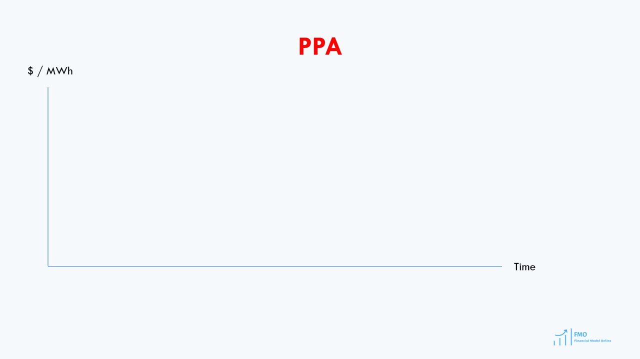 and on the horizontal axis we've got time. In physical PPA, the energy price is fixed and this is represented by the horizontal line which does not change over time. In the vertical axis, we've got time and on the horizontal axis, we've got time. 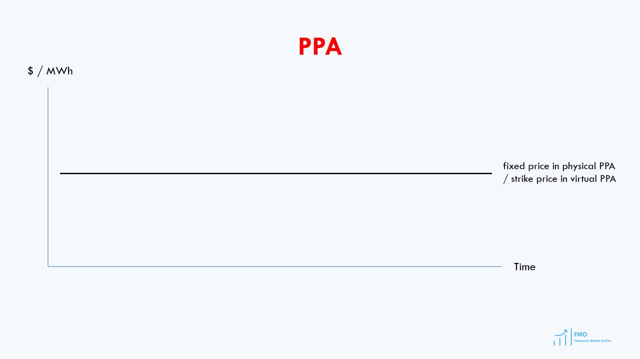 This is also true for virtual PPA. However, the fixed price is usually referred to as the strike price. Next, we've got the market price of energy, which is fluctuating, And in this example, it's fluctuating around the fixed price, which may or may not be the case in real life. 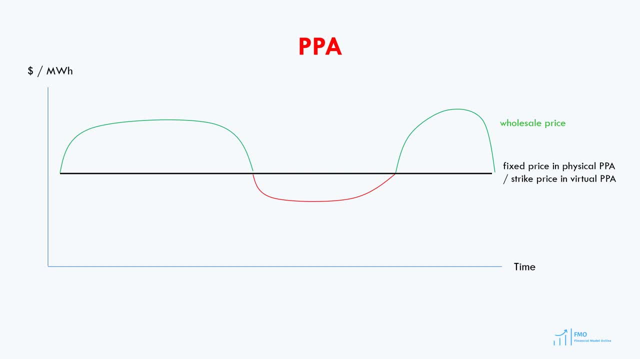 So the market price is relevant for the virtual PPAs, because remember that the virtual PPA is a contract for difference. When the market price is above the strike price represented by the point B on the chart, the power producer will pay the difference between the market price and. 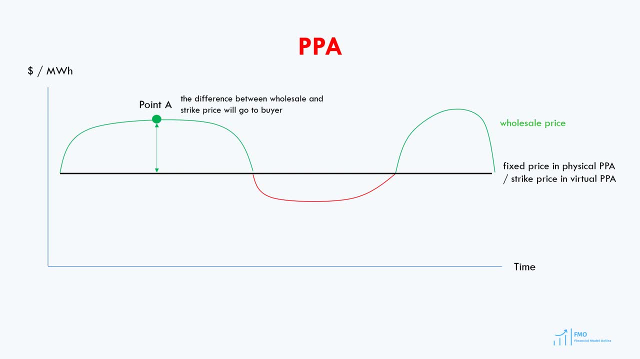 strike price to the power purchaser. Remember that under virtual PPA, energy is sold to the market rather than power purchasers directly. The same is true when the market price of energy is lower than the strike price. In this case, the power purchaser will compensate the power producer for. 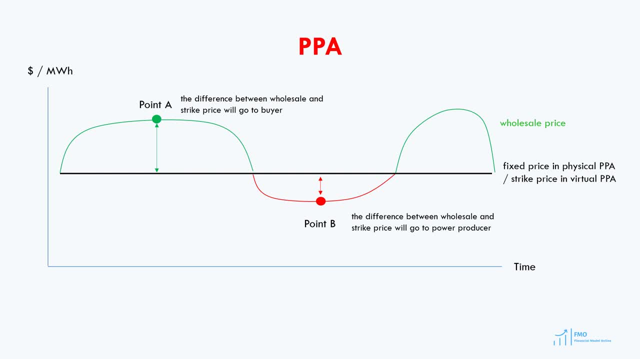 the difference between the market price and the strike price in the PPA. So this is how the example is: a fixed price PPA and it's fixed during the whole PPA tenor. This type of fixed pricing is common in the US market. However, the fixed price can also be escalated according to: 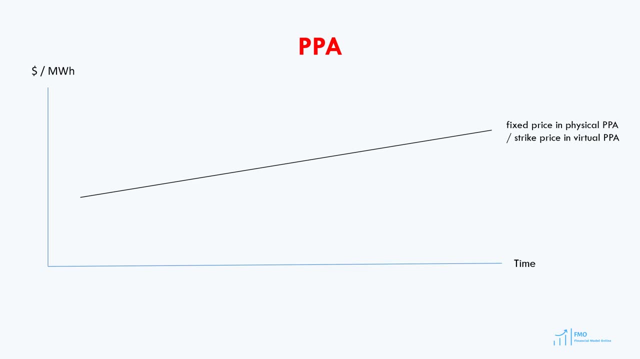 some formula such as a 1% escalation per year, or the price can be tied to an index, such as CPI index in the US. In such cases where the price is escalated, the price in the PPA will be upward sloping and then we will have the fluctuating wholesale price around the PPA price. 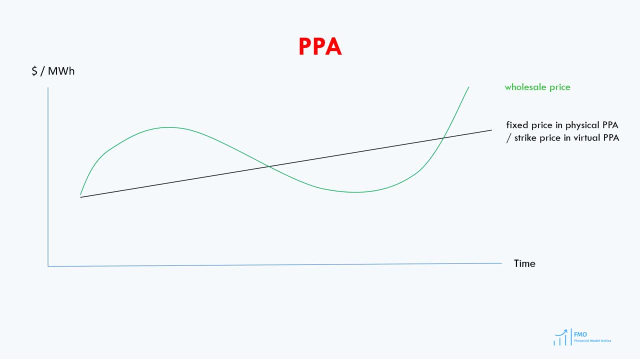 So both the fixed price and escalating price are more or less well-known in the US and other markets worldwide. Another pricing scheme we see in power projects, which is common in coal-fired or gas-fired power projects, is a two-part or two-level tariff In this type of tariff structure. 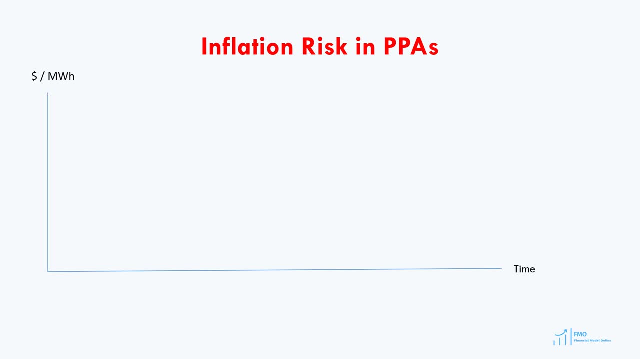 we usually have a tariff that covers the capital cost and another tariff that covers the operating cost component. This type of tariff is popular when we need an inflation hedge, For example, if we have a tariff that covers the capital cost and another tariff that covers the 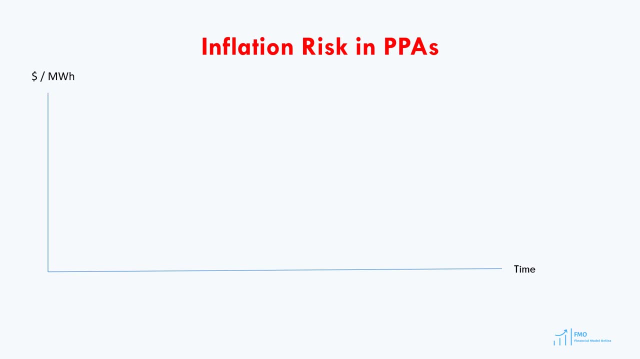 operating cost. we will have an inflation hedge, For example in a PPA where the energy price is tied to a certain index like CPI. we will have a projected revenue in our financial model that goes up over time in line with the CPI index and this is represented by the upward sloping. 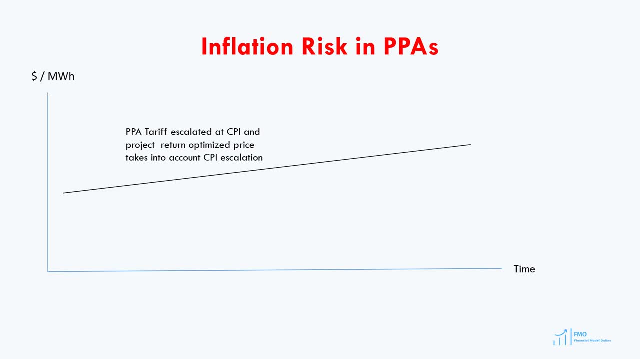 line on the chart. However, remember that this is just a projected revenue based on project CPI numbers. Also, remember that in our financial model, the PPA price will be optimized for certain input parameters, including CPI, to get to the required rate of inflation. 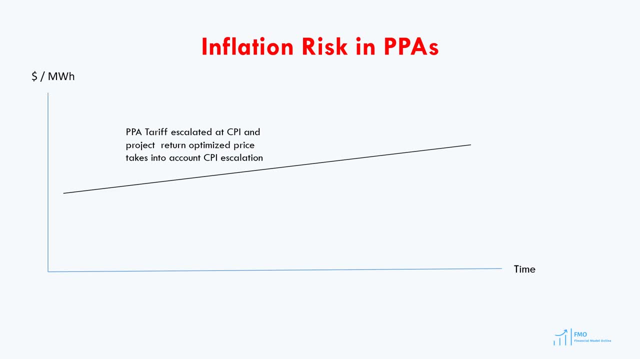 Those of you who have taken the Project Financially Modeling for Renewable Energy course are familiar with its optimization process. The question is: what happens to the equity return of the project if the realized CPI is less than the projected CPI? In such a case, actual revenue will be less than the projected revenue because of the lower realized. 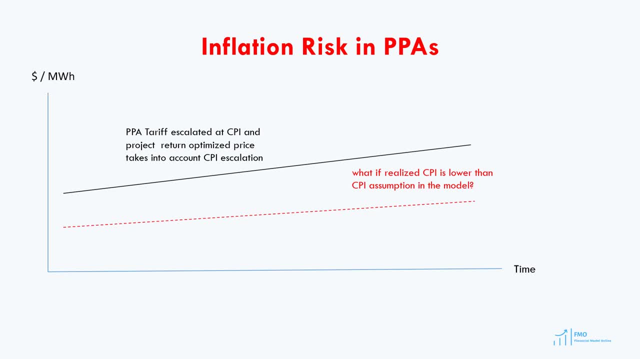 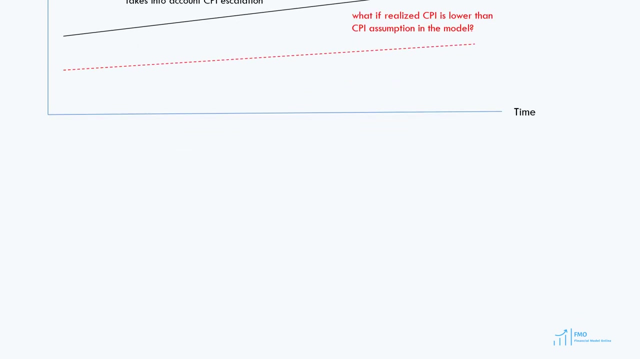 CPI number. Hence realized rate of return will also be lower than the required rate of return. Therefore, in PPA, where energy price is tied to a certain inflation index and is projected to increase every year, the power producer takes on the risk of inflation. One solution to this is to 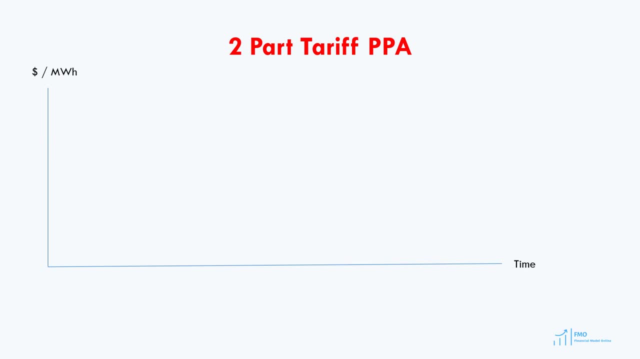 have a two-part tariff where price optimization is based on this two-part tariff. In a two-part tariff structure we will have the capital cost component in the tariff and the operating cost component. The capital cost tariff will not be tied to any indices and will be fixed throughout. 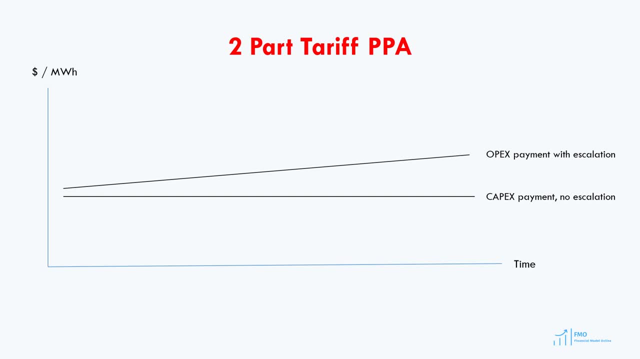 the life of the PPA. Therefore, in PPA, where energy price is tied to a certain inflation index and is fixed throughout the life of the PPA, this tariff will include the debt service and equity return to the investors. The second tariff is the operating cost tariff and will be linked to the 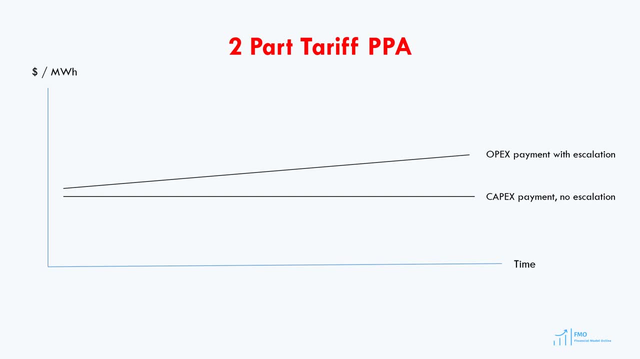 same index as the index used to escalate operating costs. So under this structure, even if the actual CPI is less than the projected CPI, the project's equity return is now hedged against inflation, because the equity return component does not depend on the projected and realized inflation. 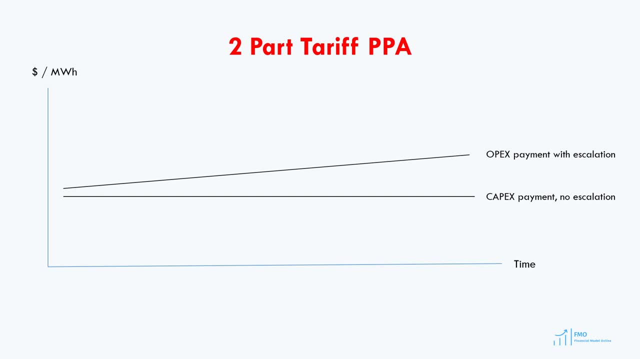 Remember that this is accomplished through price optimization In the model where only the operating costs tariff is escalated while the capital cost component is kept fixed. So it's important to remember that you might sometimes see this two-part tariff structure, which is not common for renewable energy projects in North America or 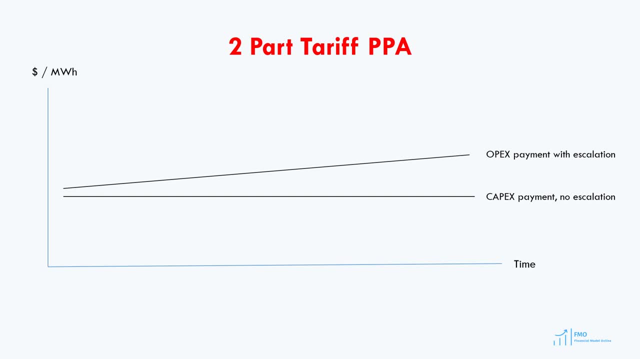 Europe, but you may encounter it in other parts of the world. To summarize, we have so far reviewed the PPA pricing structures, where the price is fixed, where the price is linked to some inflation index, and also a two-part tariff structure. 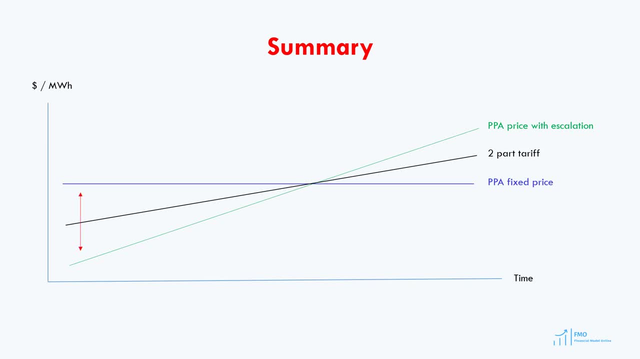 Note that under the fixed pricing structure, the payments in the early life of the project are higher than the payments under the PPA pricing with escalation. This means that the power producers get paid more upfront in the fixed pricing structure, which is usually what equity. 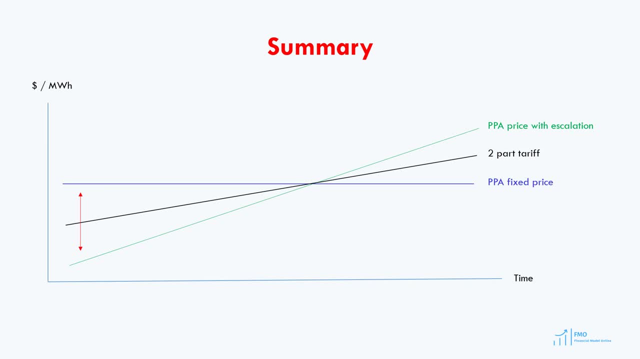 investors and lenders want because the project's debt is paid off faster under the fixed PPA price structure. And finally, we saw that under the two-part tariff we are hedged against inflation and the actual or realized inflation compared to the current tariff with the PPA price structure. 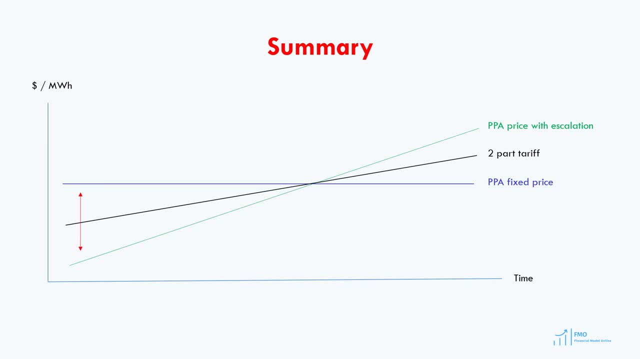 to the projected inflation will not impact the equity returns. Sometimes we might encounter a pricing mechanism where the price is linked to the wholesale market price, offering a discount. In these cases, there is a predetermined fixed PPA price that acts as a floor price. and then we've got a fluctuating wholesale price. Since the PPA price offers a discount to the market price, our price under the PPA will always be lower than the wholesale price. As such, when the wholesale price increases, the PPA price follows suit, and vice versa. 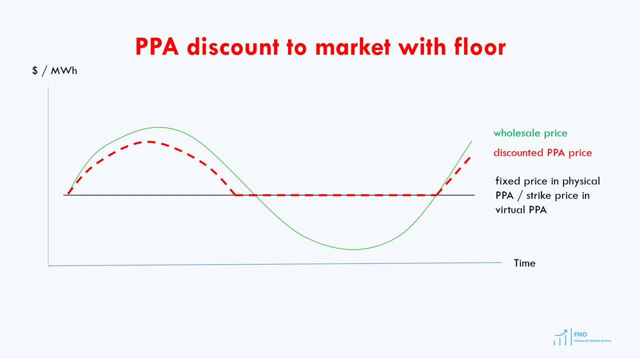 when the market price decreases, the PPA price will also fall. However, the PPA price can only decrease up to a certain limit due to the established floor price. An alternative pricing structure is when the price is linked to the wholesale market price. However, there is both. 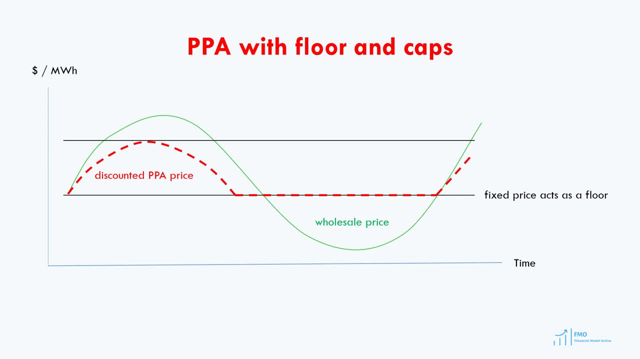 a floor price and a ceiling or cap price. In this case, both the downside and upside PPA price movements are limited. The PPA price will fluctuate within a specified range. We may also encounter a pricing structure where a portion of the tariff is fixed. 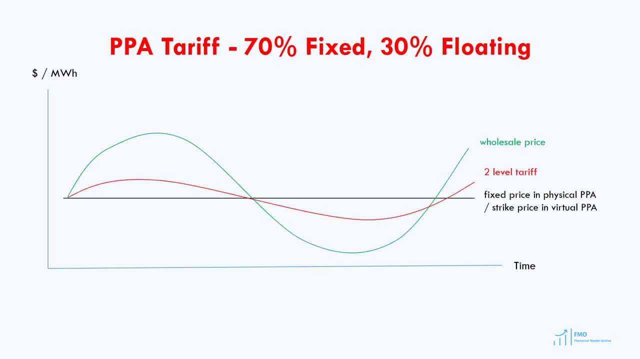 and another portion is linked to the wholesale energy price. For example, it could be specified in the PPA that 70% of the tariff is fixed, while 30% is linked to the wholesale price. The PPA price in this structure will fluctuate between the fixed and wholesale prices. 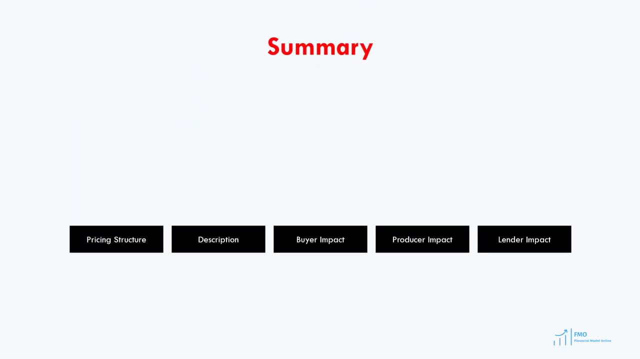 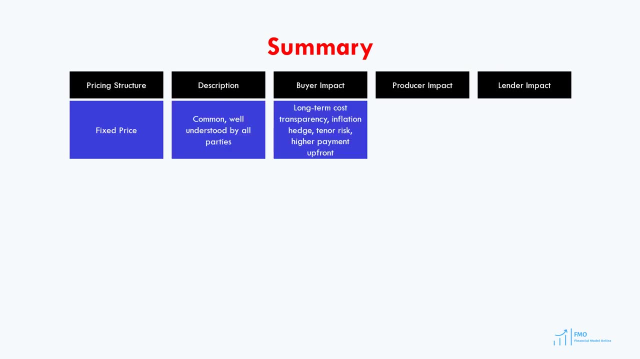 In summary, the different pricing mechanisms under various PPAs include the fixed price, which is common and well understood by market participants. Buyers who sign these PPAs have transparency in energy costs. They know exactly how much they have to pay and for how long. A fixed price provides an inflation hedge. 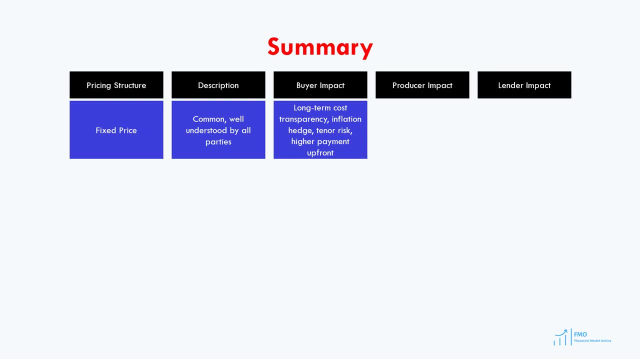 but it also exposes the buyer to long-term tenor risk should the wholesale price be lower than the fixed price for a substantial period. The buyer also faces higher upfront payments under fixed price PPA compared to prices under PPA prices with indexation, as we saw earlier From the power.